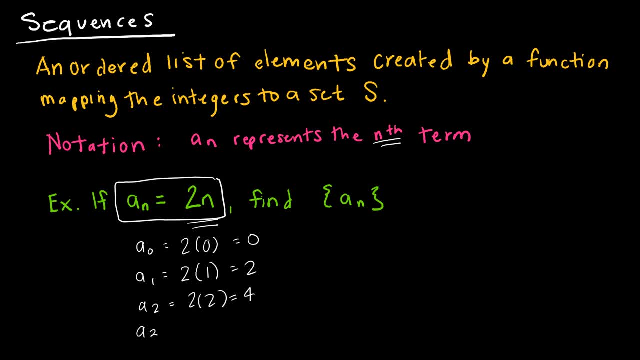 Which is 2 times 2,, which is 4.. a sub 3, which is 2 times 3,, which is 6.. And we can see that if they're asking me to find the set of values that create the sequence, 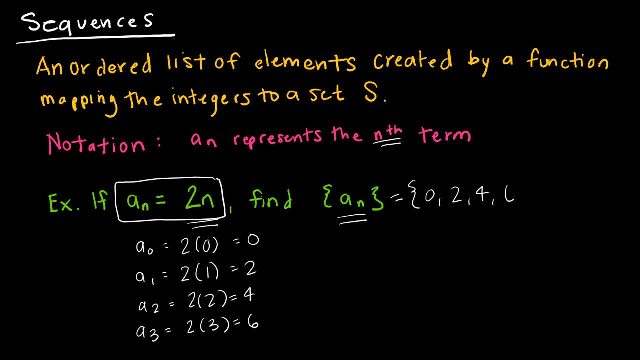 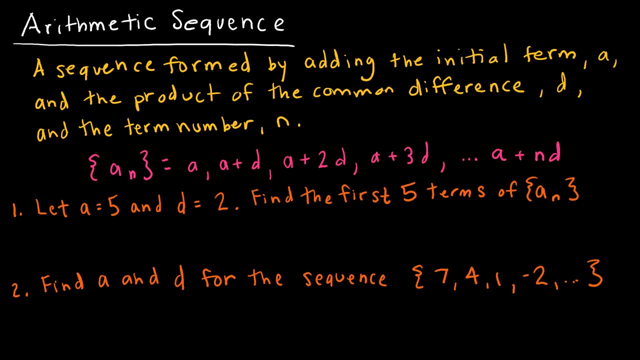 that would be 0,, 2,, 4,, 6,, and this pattern would continue. We're going to look at two types of sequences in this video. The first is the arithmetic sequence that is formed essentially by adding some common difference, starting with some initial term. 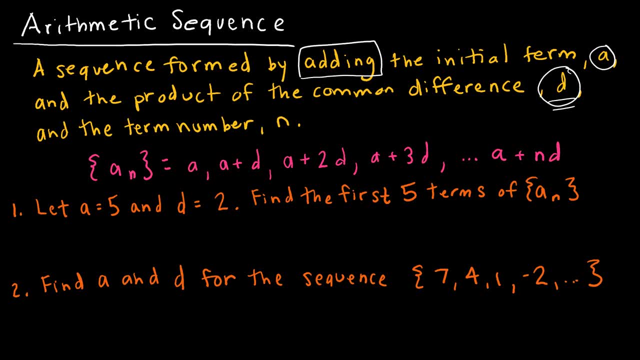 And we're just going to keep adding that common difference n times. So let's take a look at what that means before we do any practice. My first term in the sequence is, whatever they tell me, it is the initial term a. To get to the next term, I'm just going to add d. 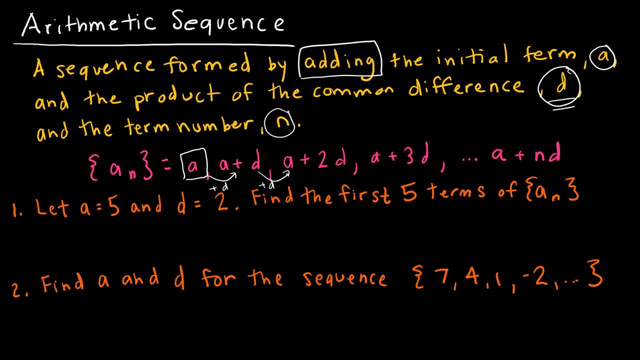 And then, to get to the next term, I'm going to add d again. or I could have just added 2d to my initial term And then, to get to the next term, I'm going to add 2d And then, to get to the next term, I'm going to add 2d again. 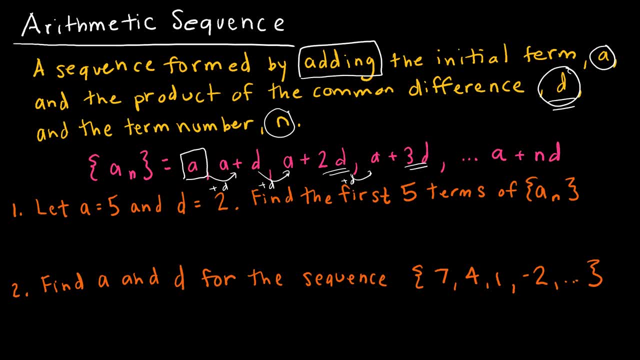 or again, I could have added 3d to the initial term, And we can see that that pattern is going to continue and we're just going to have n d's added to the original. Now why is this important? Because in arithmetic sequence we can either just use the initial term. 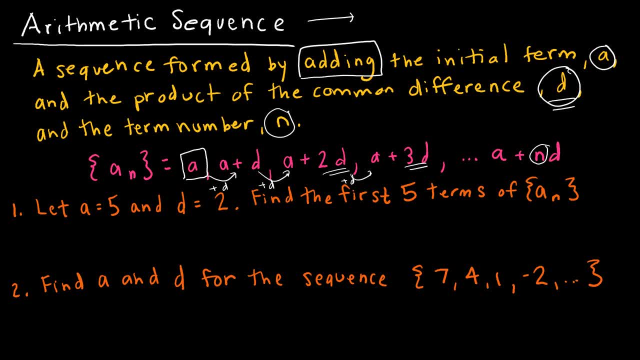 and the common difference, to find values in the sequence, or we can write it explicitly, And explicitly means I can write an equation and I can write an equation and I can write an equation where all I have to do is plug in n and to find whatever term I want. 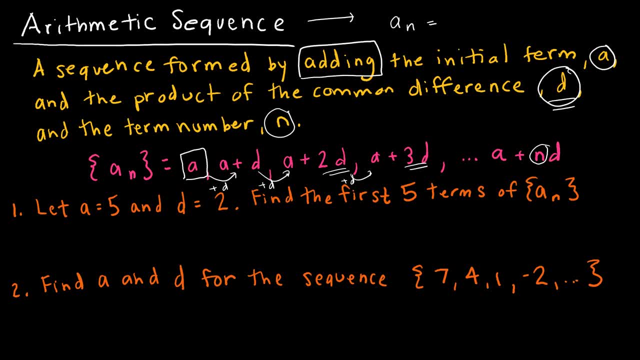 So, for instance, a sub n in this case, well, in any case would be a plus d, n or n d, It doesn't matter which one comes first. So this is how you write an arithmetic sequence. explicitly, Remember this, because it's not going to go away. 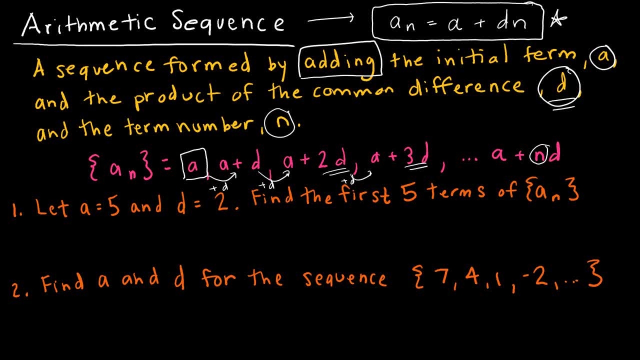 and when we talk about recurrence relations, we're going to see why writing things explicitly is so important. For our first question here, number one, they've given me a and they've given me d, So if I want, I can go ahead and write this as a sub: n is equal to 5 plus 2n. 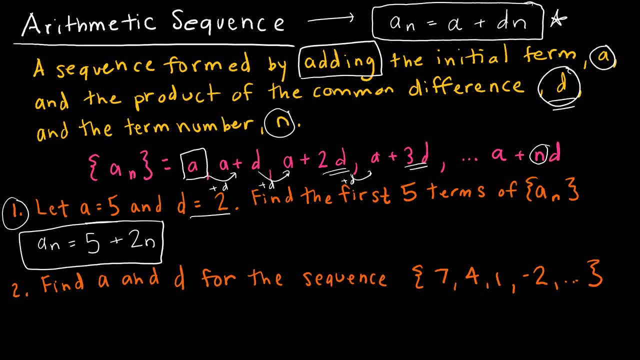 This is how I would write this explicitly If I wanted to find, answer this question and find the first five terms of the sequence. then I've got a choice. I can either. I mean either way. I'm starting with 5,. 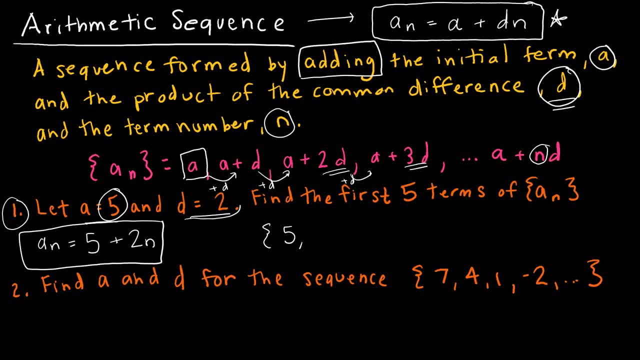 because that's my initial term. If I want, I can then just use that common difference of 2 to say: okay, to get to the next one, I'm just going to add 2, and then, to get to the next one, I'm going to add 2,. 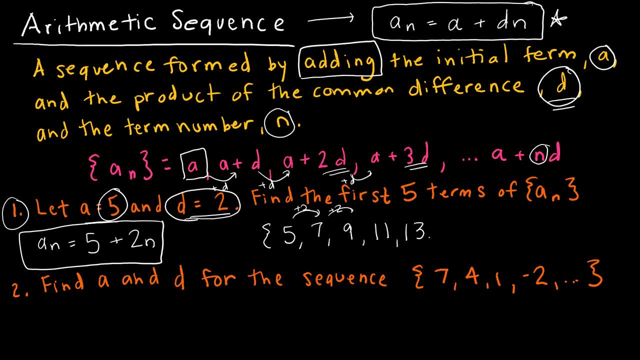 and then to get to the next one, I'm going to add 2 and add 2, and we can see this pattern would continue. So what we've done there is essentially a recurrence relation, and that's our next video- is a recurrence relation. 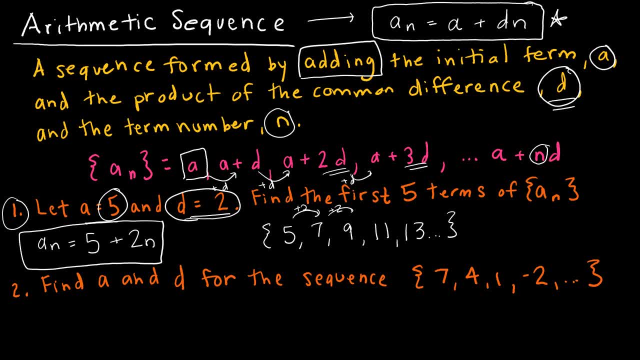 but I just want to point out to you the difference. now A recurrence relation says: take something that you have before it and do something to it to get the next term. An explicit function doesn't need the term before it. So let's say this was a sub 0,, this was a sub 1, a sub 2, a sub 3, a sub 4.. 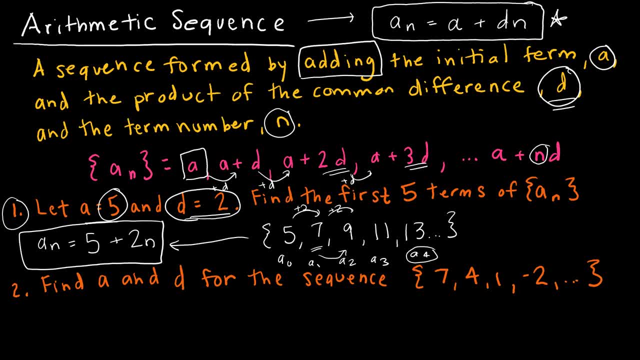 So let's find a sub 4. using my explicit function, a sub 4 would be 5 plus 2 times 2.. So let's find a sub 4. using my explicit function, a sub 4 would be 5 plus 2 times 2.. 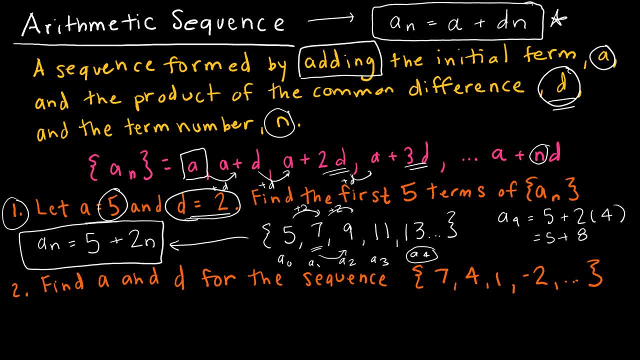 2 times 4 is 8.. 5 plus 8 is 13.. Notice, I got 13,, the same as I got when I wrote it out recursively. So again, you might not quite get the recursively and explicitly yet. 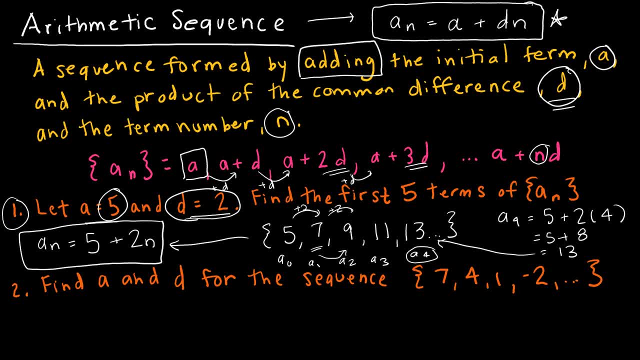 We're going to focus on that in the next video, but this is just a good precursor to that. The second question says: find A and D for the sequence. So again, it's not necessary for us to write this in the explicit form, but it's not a bad idea to get the practice. 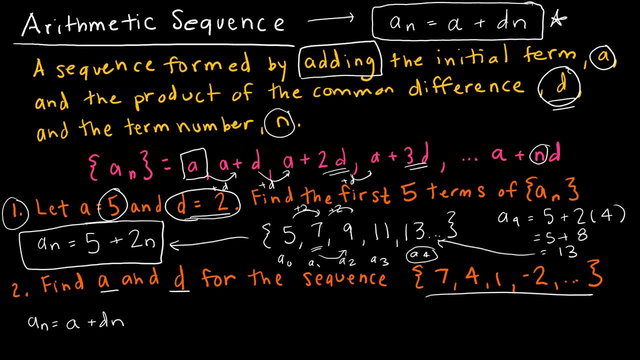 But we're saying: hey, we don't have A and we don't have D, Here's a sequence, figure it out. So 7, obviously is my first term. A must be 7, which means over here A would be 7.. 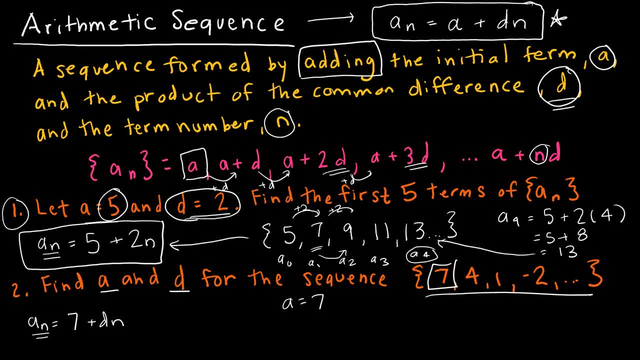 Notice I'm not doing anything to the left side. We keep that so that we understand. that's how to find the nth term. Now I have to find the common difference, So here I'm going to take the term before it. 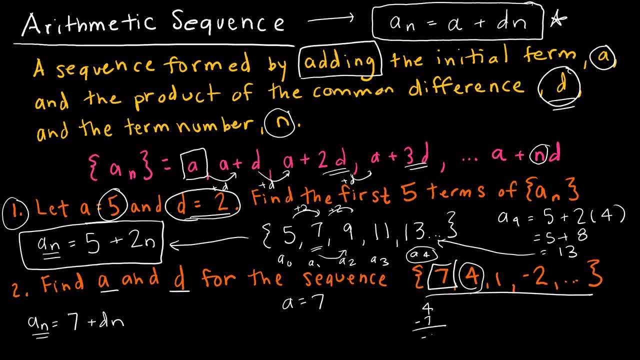 and subtract the first term, and whatever I get is going to be my common difference. Now I could do that again. I get a common difference of negative 3.. I could also say 1 minus 4, also negative 3,. 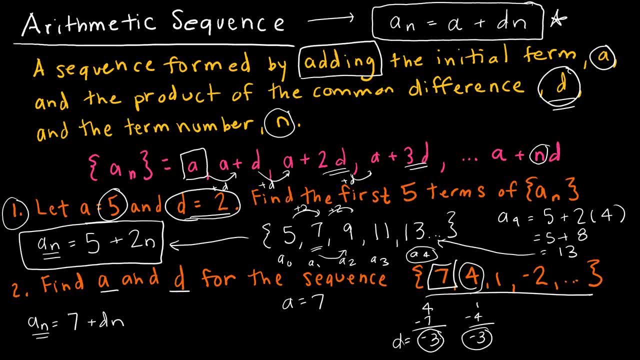 and that should be the same all the way through, Otherwise it's not an arithmetic sequence. So here we have just found D is negative 3. Again, by taking a term before and subtracting the previous term. so now, if I wanted to write this explicitly: 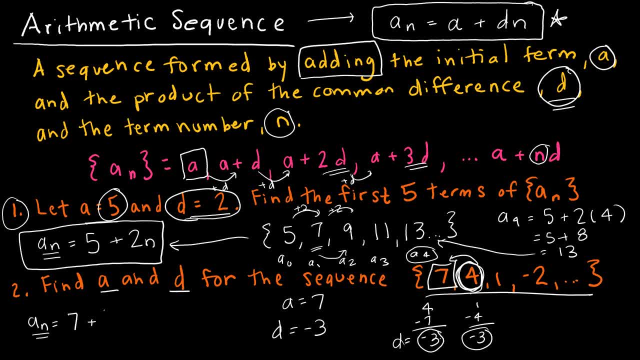 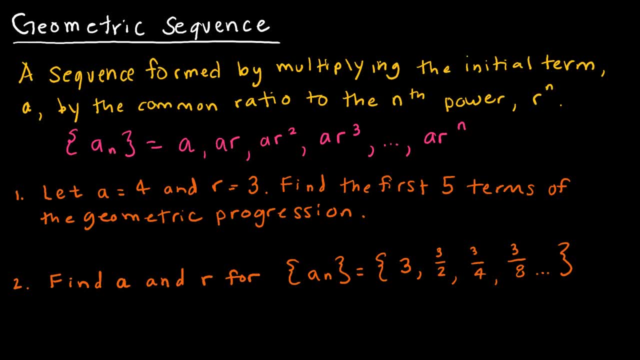 I could write negative 3D. The other sequence we want to take a look at here is the geometric sequence, and a geometric sequence is different from an arithmetic sequence because in an arithmetic sequence we were adding and in a geometric sequence we are multiplying. 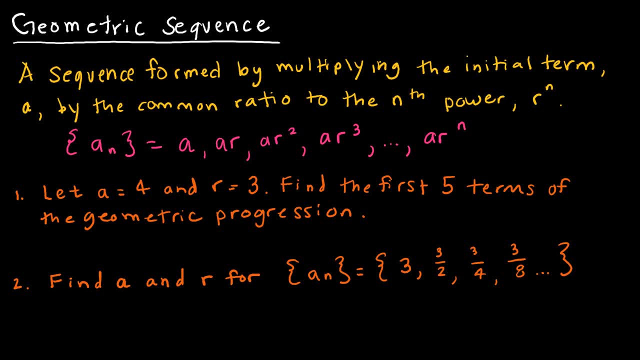 So, just like we did in our last example, we want to take a look at the geometric sequence and we want to know how can we write this explicitly because, again, that's going to be super important moving forward. So let's take a look at what the geometric sequence is all about. 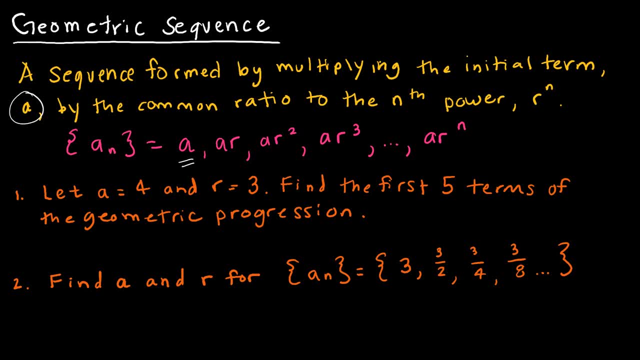 We start with some term A, so that's what we're familiar with- and then we're going to multiply by some common ratio which is R, and we're going to do that n times. So here I'm going to take. 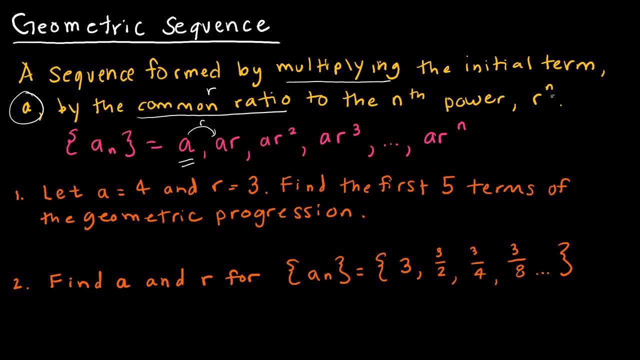 A times R to get AR. Then I'm going to multiply by R again, or remember: that means I've essentially multiplied my initial term: times R twice, or R squared- Not 2 times R, but squared- And then times R again. 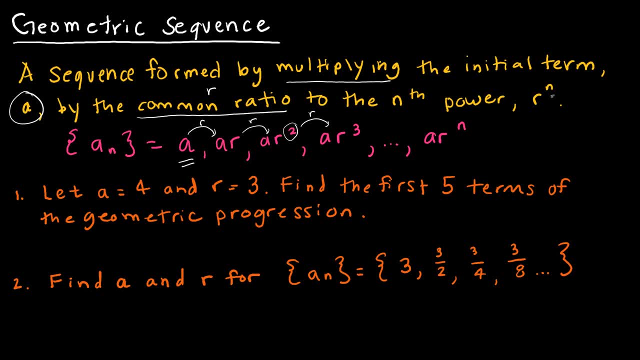 so now I've multiplied by 3Rs and then times R and times R, and I'm doing this n number of times. So if you need to write a geometric sequence explicitly, A sub n would be A times R to the n. 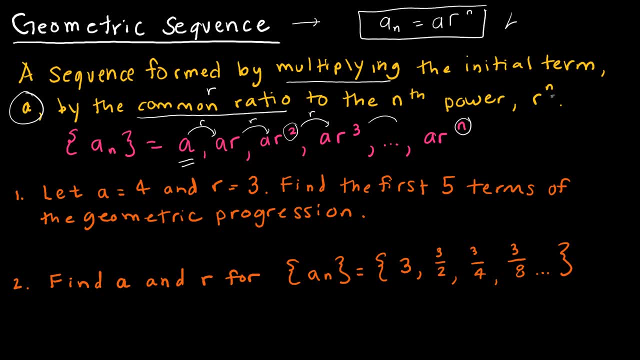 So again, remember this, because it's not going to go away. you're going to use it a lot. So let's take a look at the two types of questions. Again, here they're telling me A is 4,. 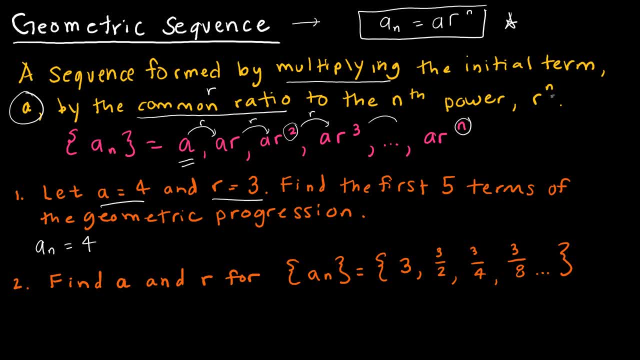 and n or R is 3.. So it's 4 times 3 to the n. Now, just as I did before, I can either look at this recursively by taking whatever the term was before it, or I can look at the explicit definition. 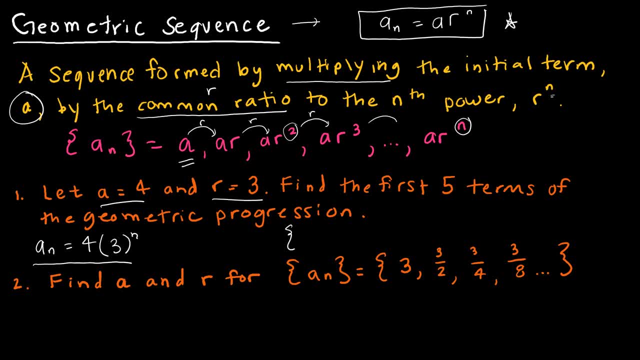 So if I want to find the first five terms- my first term is 4, and that's considered A sub 0, because it's the initial term- And then to find the next term, if I'm doing it recursively, I'm just taking this 3 and saying: 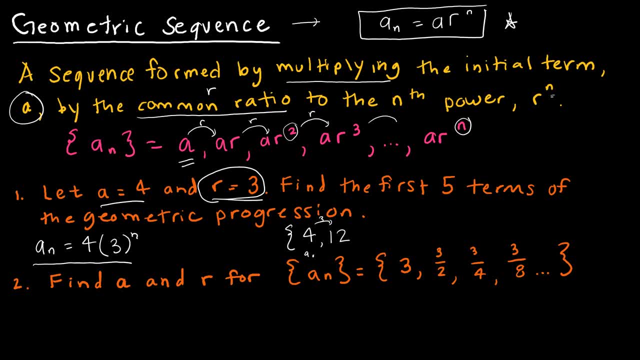 well, I'm going to multiply by 3 to get 12.. And then I'm going to multiply that by 3 to get 36.. And then I'm going to multiply that by 3 to get 108, and that by 3 to get 324.. 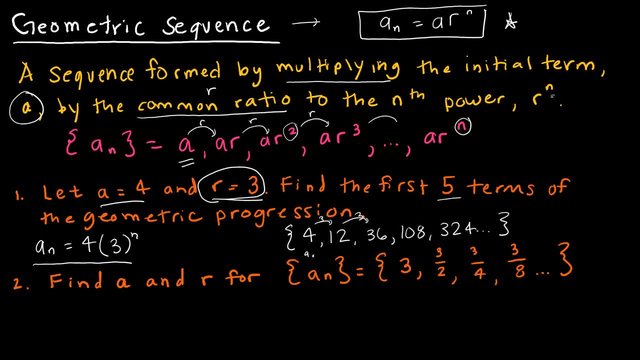 And that's all I have to find, because they said first five terms. The other way that you can do this again this would be A sub 1, A sub 2, A sub 3, A sub 4.. The other way that you can do this is, of course, 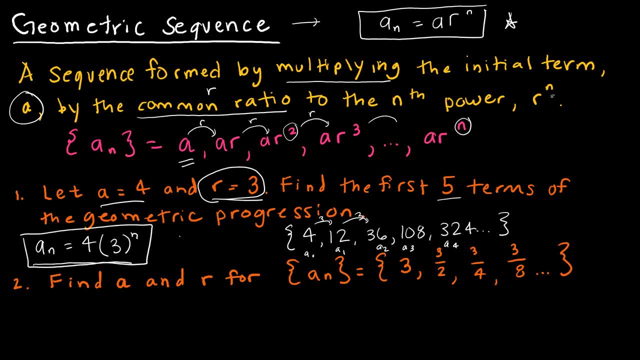 use this explicit definition. So let's look at A sub 3.. According to my definition, it says 4, times 3, to the third. Well, 3 to the third is 3 times 3 times 3,. 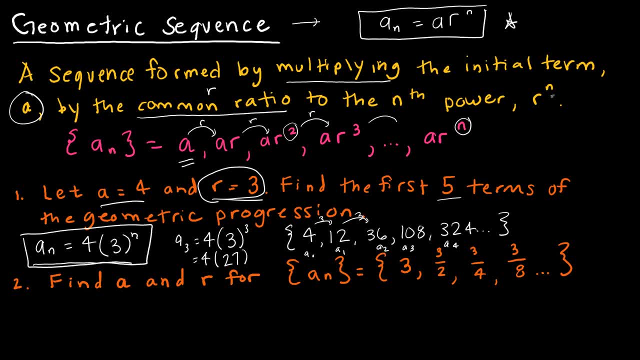 or 27.. And 4 times 27 gives me 108.. So we can see that whether I did it recursively, just by multiplying the term before it by 3, or using this explicit function, I'm going to get the same answer. 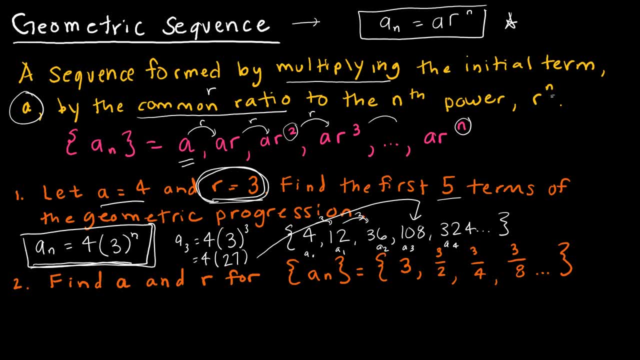 For my second question, again I have find A in R, and here's the sequence. So how are we going to go about this? Well, again, A is very easy to find. So over here we're going to build our A? R to the N. 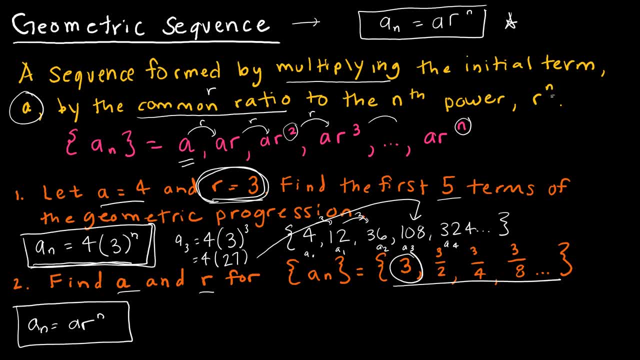 because you should get in the habit of being able to write it explicitly: If the first term is 3,, I'm going to replace A with 3.. And then the question becomes: how do I find the next value in the sequence? So, just as I did before, 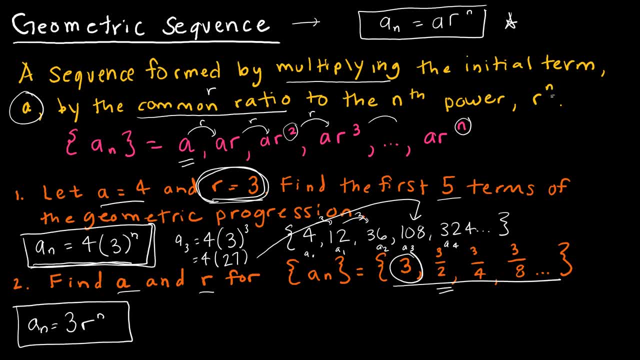 I'm going to take the next value, so not the initial, but the next value, 3 halves, and I'm going to divide it by the term before it. So in the last one we subtracted and of course we subtracted. 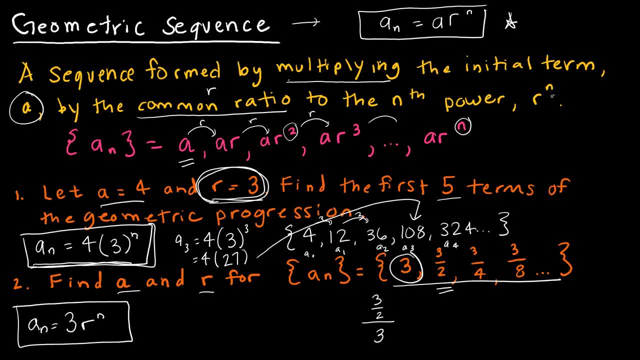 because that's the opposite of addition. In this term we're going to divide, because that's the opposite of multiplication. So 3 halves divided by 3, a lot of people freeze up when they have fractions- 3 halves divided by 3. 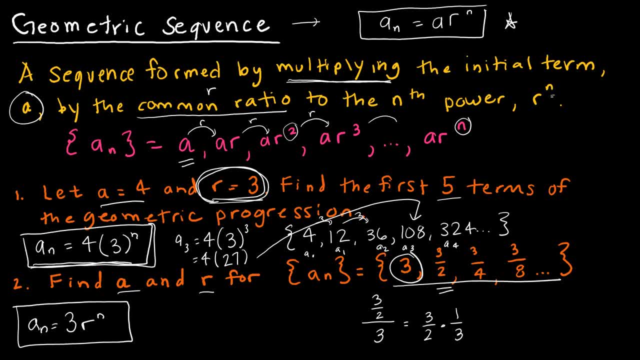 is the same as 3 halves times 1. third, Remember: I can multiply by that reciprocal, which means I get 1 half. 1 half is R, my common ratio. Now, whenever you have a common ratio that's less than 1,. 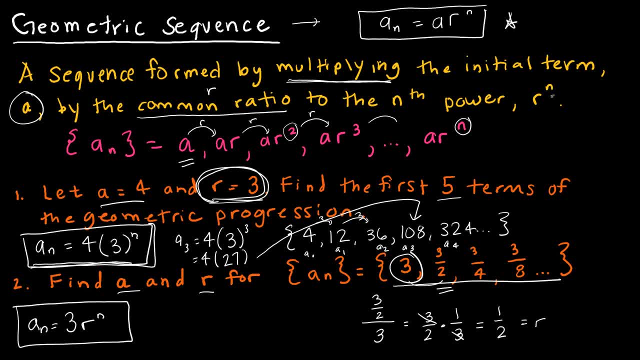 that's when you're going to get something where the terms decrease. So if it's between 0 and 1, that's when you're going to get a decreasing sequence. But what I've found is R is 1- half, and so I could rewrite this. 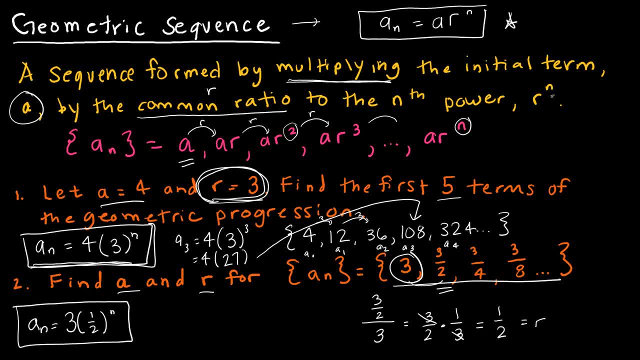 as 1 half to the n. Now, I know that you know this already, but just to be safe, remember that when I write it like this, the 1 half is the only thing that goes to the nth power. So that 4 right here. 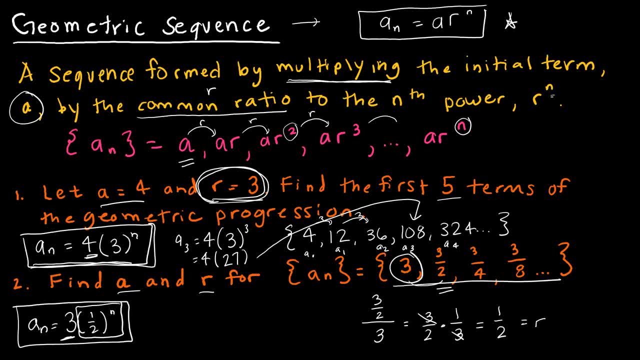 isn't to the nth power and this 3 right here is not to the nth power. It's just whatever. that R value is that common ratio? So again they've asked me to find A, and A was 3.. 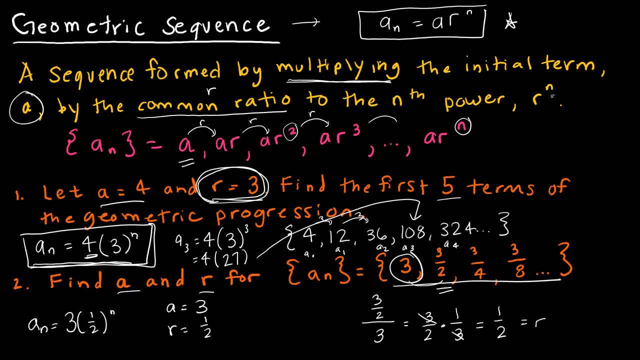 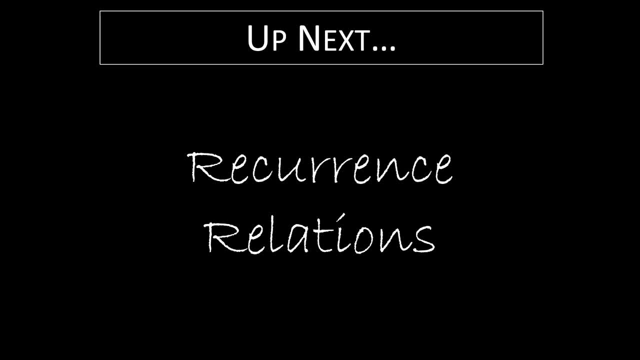 They've asked me to find R and R was 1 half, So up next we're going to explore recurrence relations in a lot more detail, And so hopefully in this video I gave you an idea of the difference between a recurrence relation. 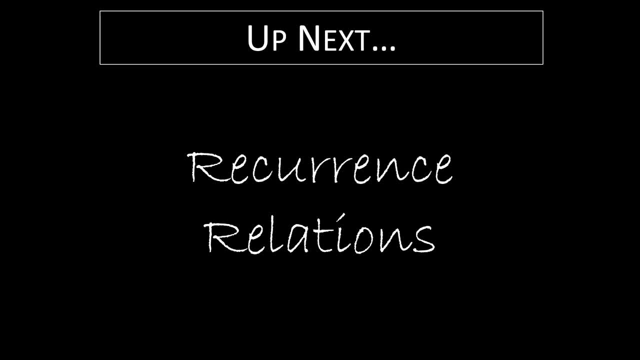 and explicit definition. But if not, hopefully I'll make it clear in the next video.